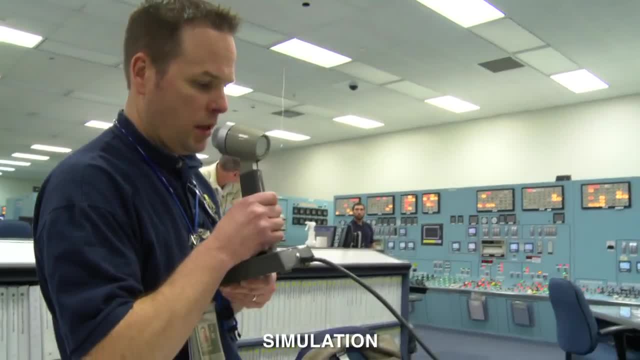 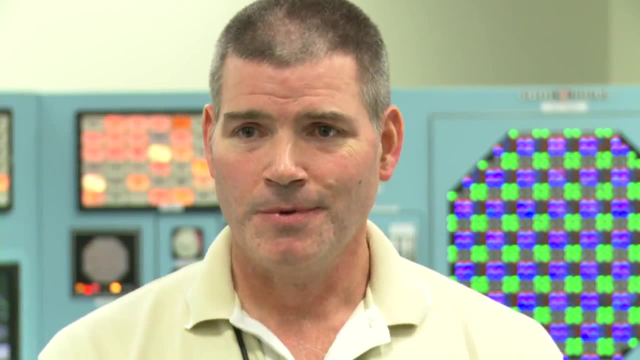 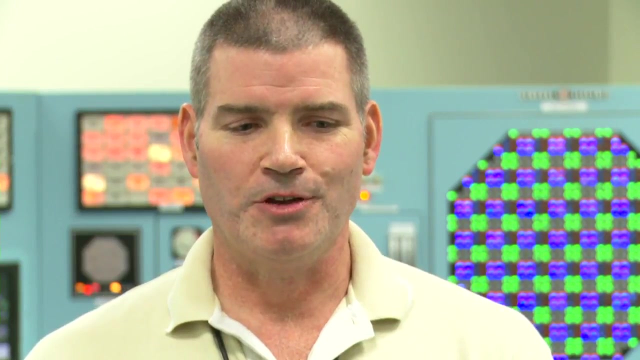 That is correct. Attention to the plant: Reactor scram due to a leak in the drywall, So it started with a leak from the reactor coolant system in the containment structure. That's what caused the initial scram, Although it would be extremely unlikely to happen. 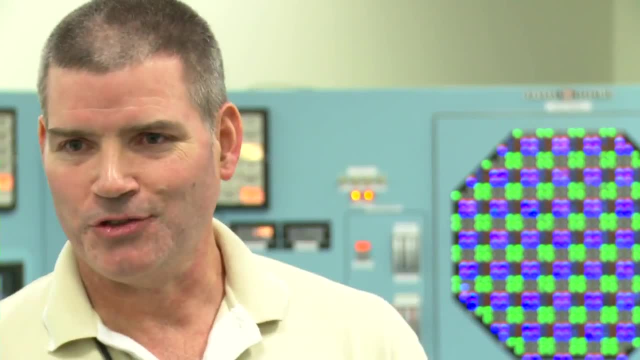 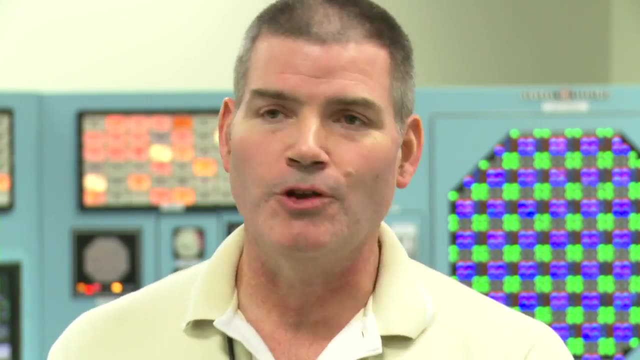 at the same time that the leak started, the two independent off-site power supplies which were referred to as the startup and the backup transformers. those were both lost. There would be no reason for those to be lost at the same time as a leak in the drywall. 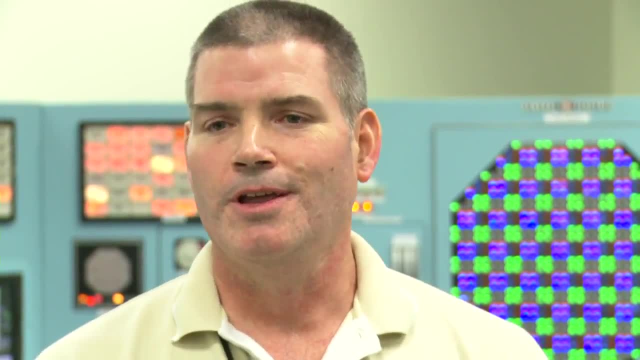 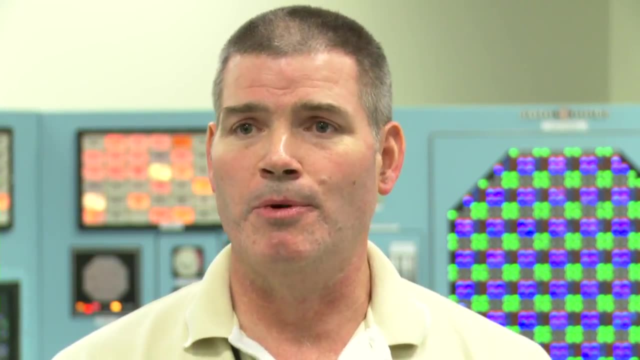 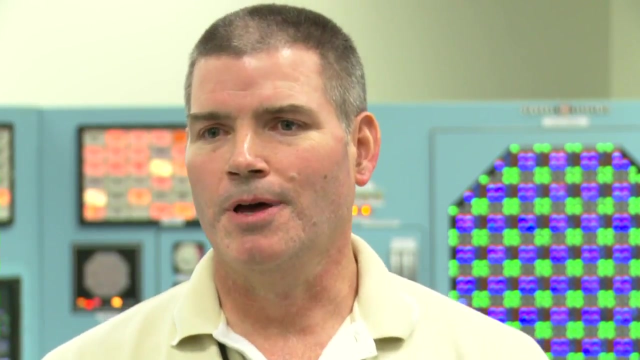 But it does take away much of the equipment that could have been used to help mitigate that leak. So with the systems that were left, which are just the bare minimum emergency systems, the crew was able to recover our PV level, keep the core from suffering any damage. 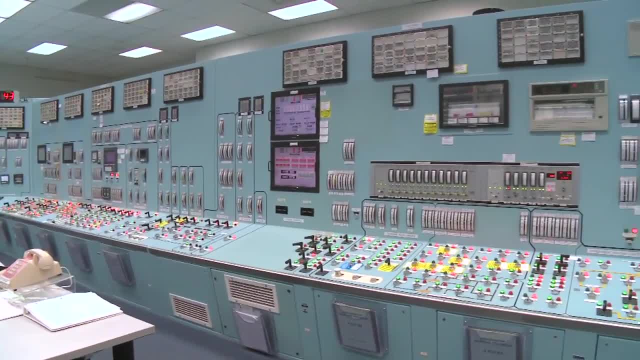 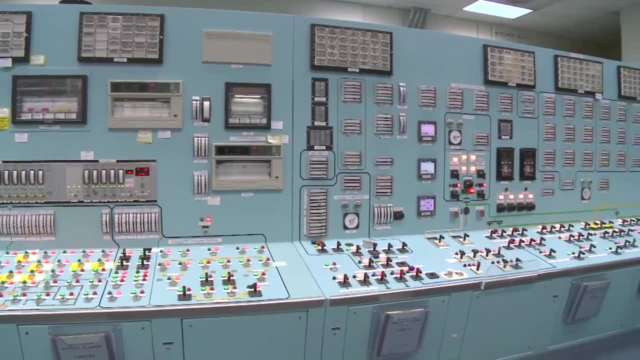 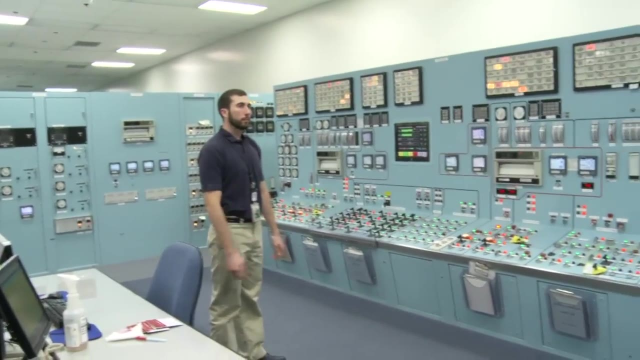 The control room simulator at Columbia Generating Station is the largest in the United States. That's because Columbia's control room is the largest in the US. The simulator is an exact replica of the control room, allowing operators to experience training and drills just as they would in the real world. 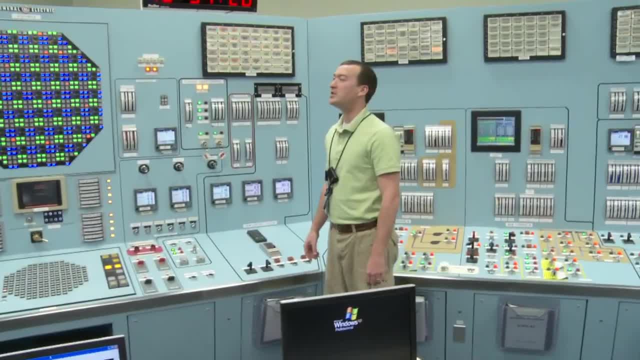 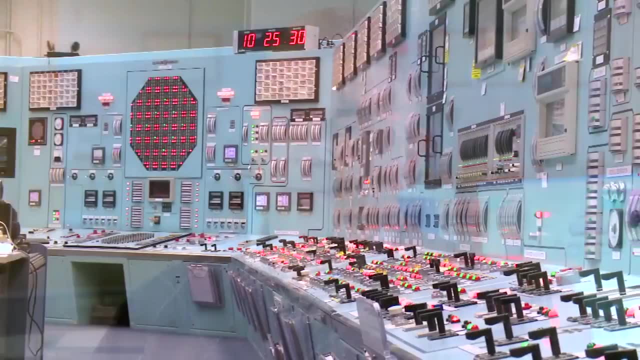 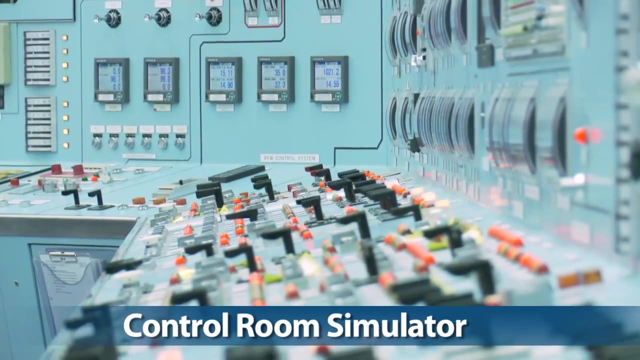 right down to the position of the wastebaskets. The NRC required that each site had a plant-specific simulator built to train their operators. on Every switch, every knob, every controller, every meter must mimic exactly the way it is in the control room. 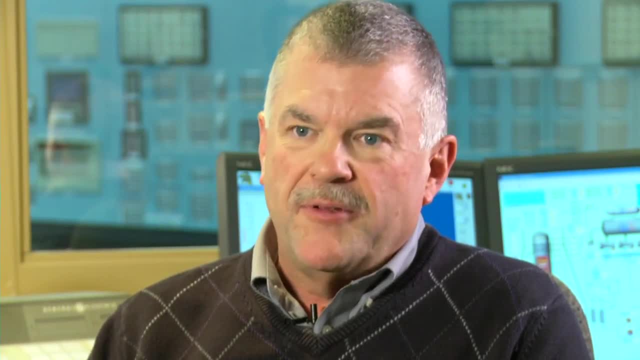 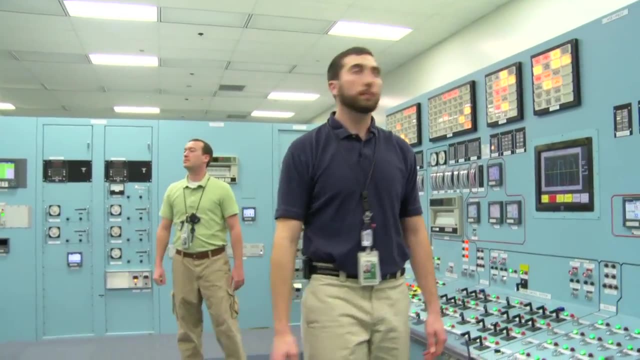 from color, to the way it feels when you operate it, to the response of the meters when you operate a system. We use the simulator for very basic type scenarios, especially when we're starting folks through their training program. We're just simple system operation. 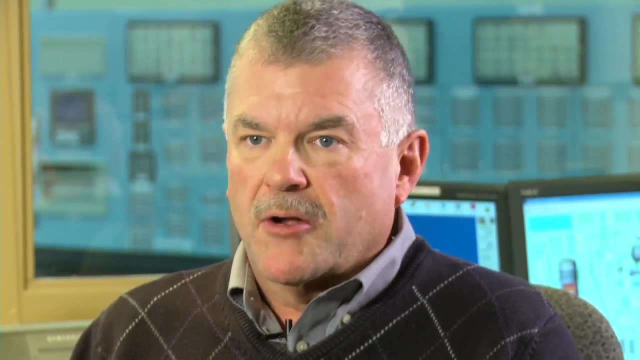 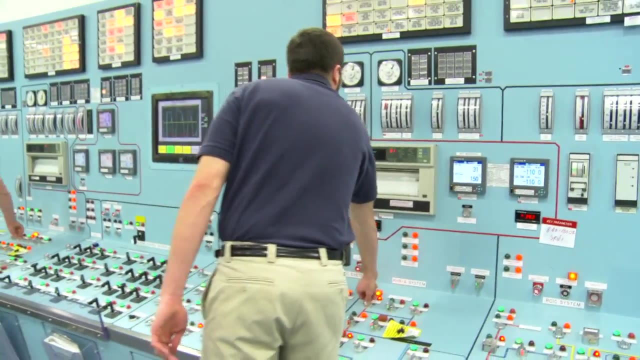 and we slowly bring them into integrated plant operation where they are able to see how operation of one particular system may have an effect on another system or another part of the plant. And then we bring them into what we call the emergency operating procedure portion of their training. 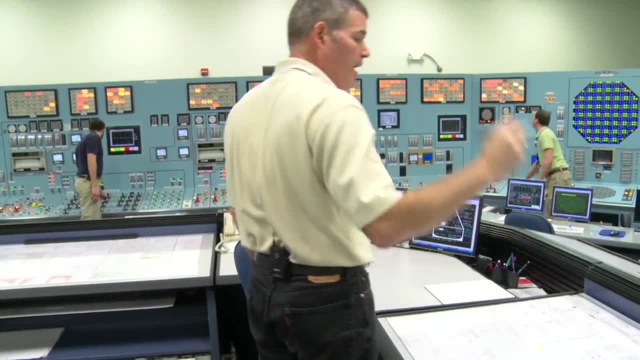 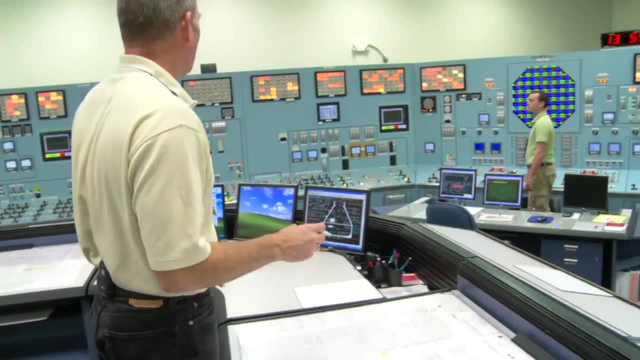 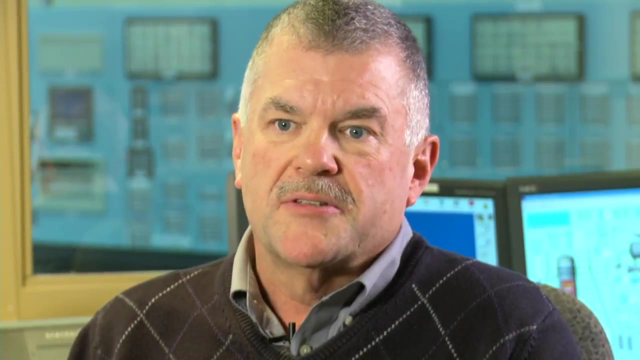 where we can run what we sometimes affectionately call crash and burn scenarios, and we take them with all different types of situations, all different types of equipment failures, to ensure that they're still able to mitigate the accident and bring the plant into a safe condition.